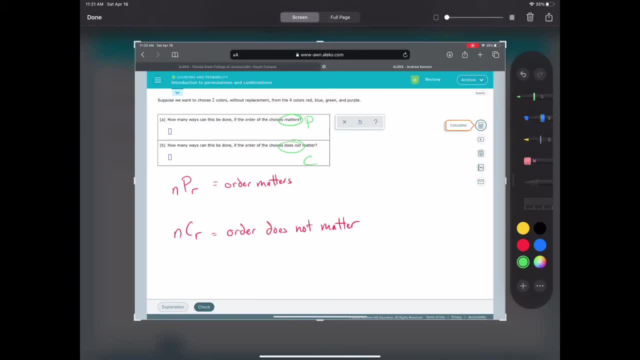 to choose two colors without replacements from the four colors red or blue. So the only way to do this is to use the combination. the order does not matter, So you just have to two numbers. to do a permutation or a combination, You need a total number and then how many you're. 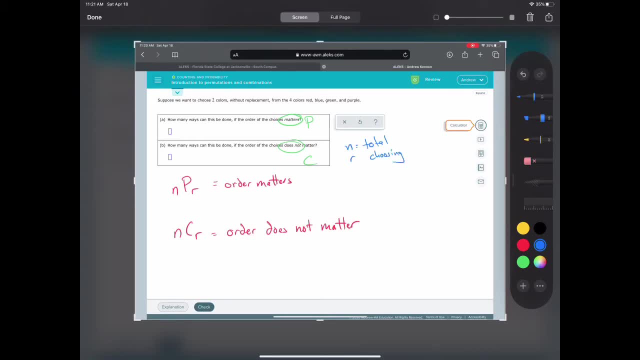 choosing. Okay, so this is your n and your r. Okay, so this would be four. part a would be 4p2 and part b is going to be 4c2.. All right, so if you were doing it by hand, you would have to do. 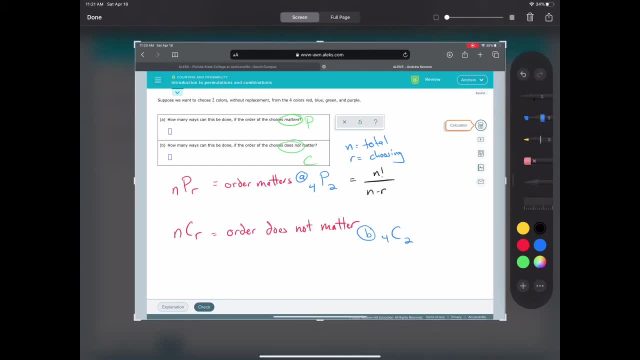 n factorial divided by n minus r factorial. So they give you these formulas and this one is n factorial r times n minus r factorial. So on part a, our n is four, because that's the total amount, and two is how many we're choosing. 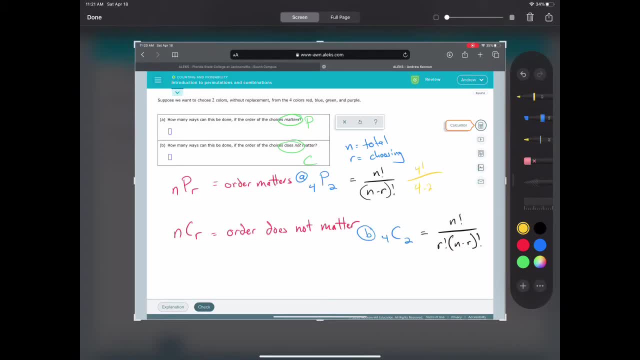 So we would do four factorial divided by four minus two factorial. So four minus two, in parentheses, this becomes four factorial divided by two factorial. You can actually just write this one out. Remember, factorial is four factorial. So you can actually just write this one out. 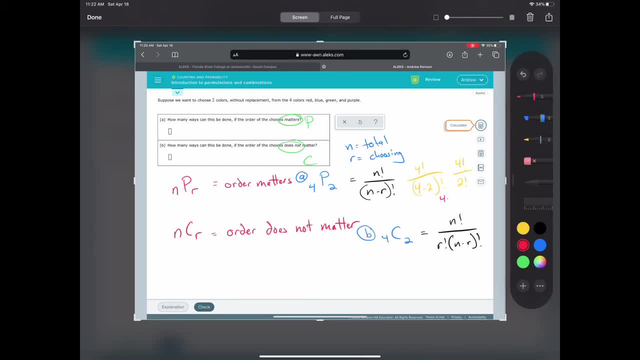 Factorial means you take that number times itself and any number less than that all the way down to one. So four times three times two times one divided by two times one. What happens here, and I show you in the example, is the two and the one cancel out, So it's really just four times. 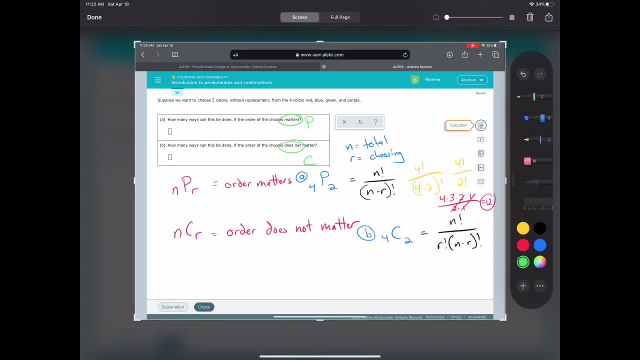 three and my answer is 12.. On the bottom one, a little more complicated, but same idea. So I do four factorial and then I have two factorial times four minus two factorial. So again, simplify, inside the parentheses That becomes two factorial. Well, okay, so again, if we write this out, it's four times three times two. 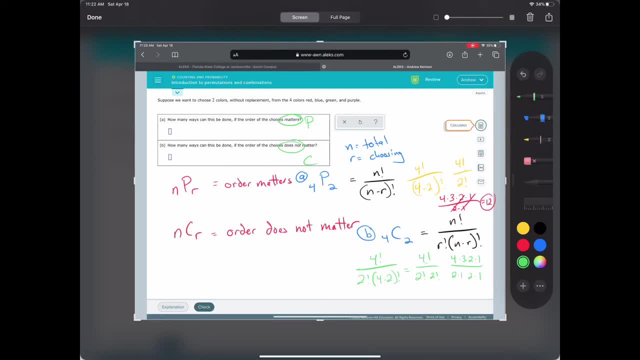 times one, and then two times one, and then two times one. So again, these cancel out. but this time I have to do 12 divided by two, which is six. So you'll always end up with more permutations and combinations, because when the order matters, you actually create more choices. All right, so that's. 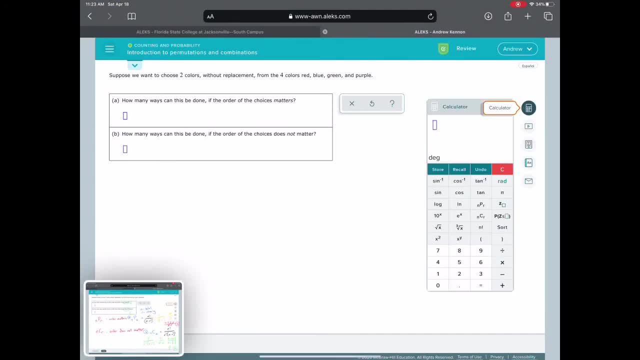 kind of how to do it by hand. With the calculator you can do it. you have a factorial button here so you could kind of double check it. So we could do like four factorial divided by two factorial, and it will do it for us. Okay, so that's one way. But if your calculator gives you,